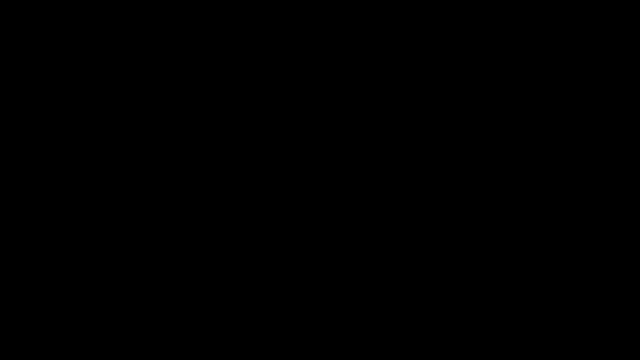 In this video we're going to talk about voltage, current and resistance, So let's begin our discussion with voltage. What is voltage? Voltage is the electric potential energy difference per unit charge. The unit for voltage is the volt. One volt is equal to one joule of electric potential energy per one coulomb. 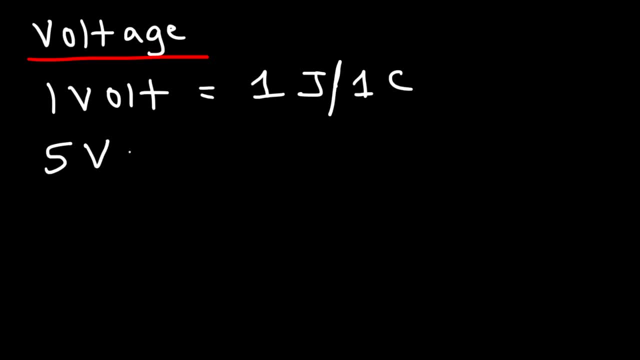 of charge. So let's say, if you have a 5-volt battery, That means that each coulomb of charge carries 5 joules of energy, or there's 5 joules per one coulomb of charge, And so the electrons, they have more energy when they're. 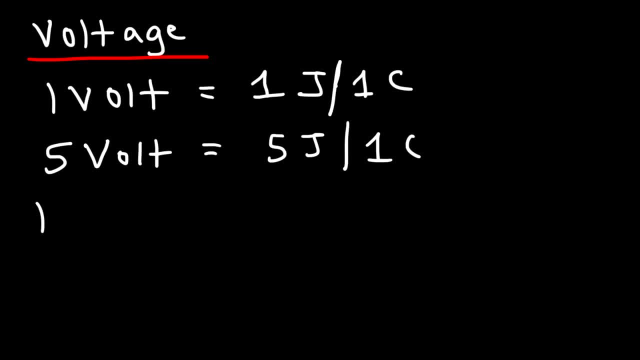 operating at a higher voltage. A 10-volt battery can pump 10 joules of electric potential energy to every one coulomb of charge, And so voltage is related to electric potential energy. Now, what about current? How can we describe current? Current represents the flow of. 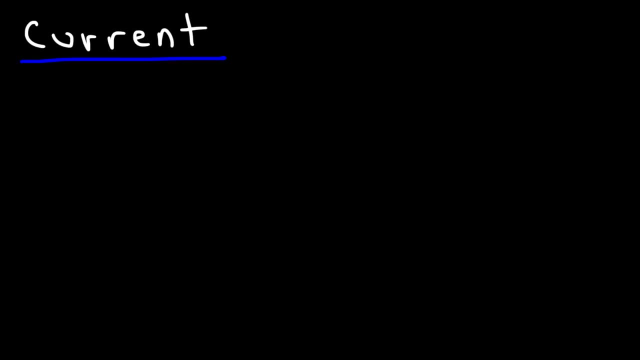 electrons. It tells you the rate at which electrons are flowing. Current is represented by the symbol i is equal to the charge divided by the time. The unit for current is the amp. One amp is equal to one coulomb of charge that flows per second. If you 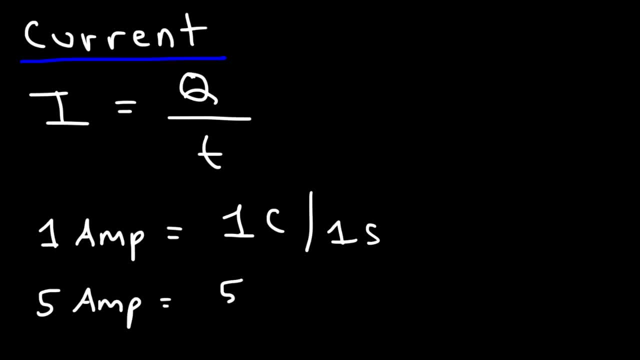 have five amps of current, then you have five coulombs of charge flowing per second. Now, when I think of current, I think of water flowing, And so water can flow very slowly or it can flow very quickly, And so you can think of that as 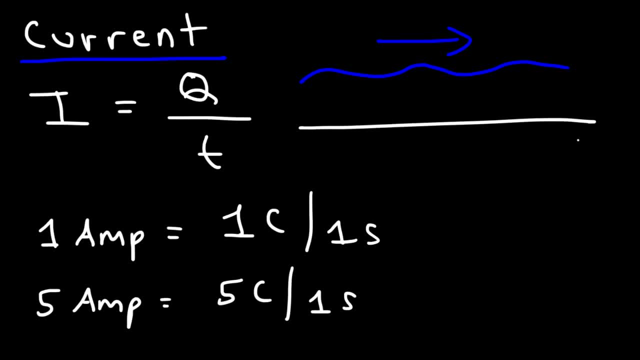 current. If you have a lot of water flowing at any given point, the current is high. If you have a small amount of water or trickle flowing through, then the current is low, And so electric current and the flow of water they have some. 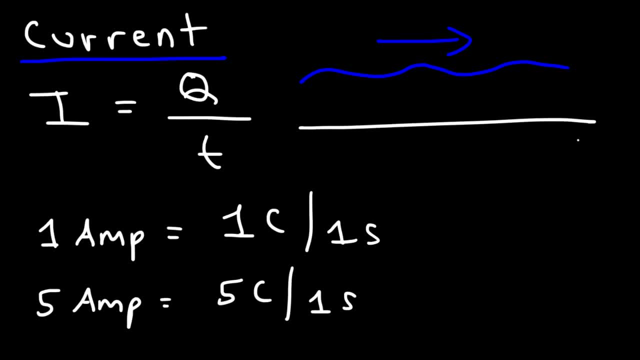 current. If you have a lot of water flowing at any given point, the current is high. If you have a small amount of water or trickle flowing through, then the current is low, And so electric current and the flow of water they have some. 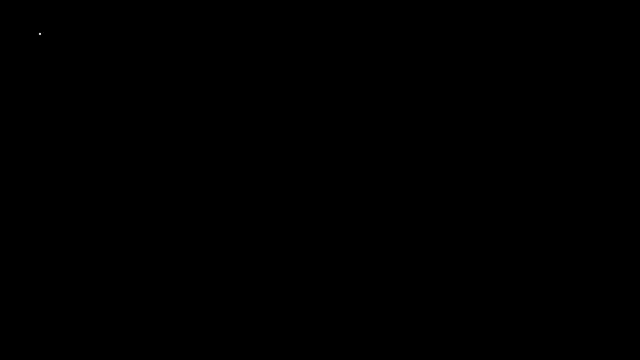 similarities in that instance. Now the next topic we have is resistance. And when you think of resistance, what do you think of Resistance? they can be used to provide a circuit by something called, or devices called, resistors, And they resist the flow of current. Resistance is measured in the unit's ohms, represented by the Greek. 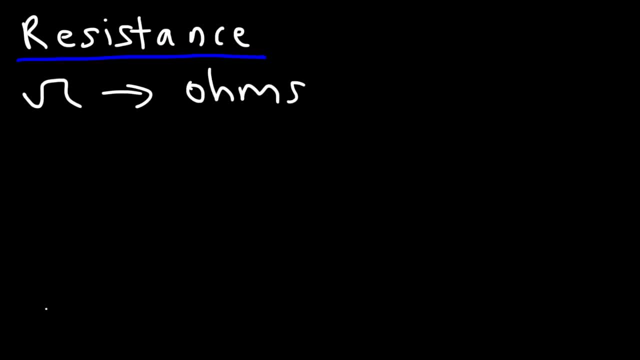 symbol omega, And that's basically what you need to know about resistors. They resist the flow of current. Now here's a question for you: Which type of wire will have more resistance? Let's say, a long wire or a short wire. What type of wire will have more resistance? 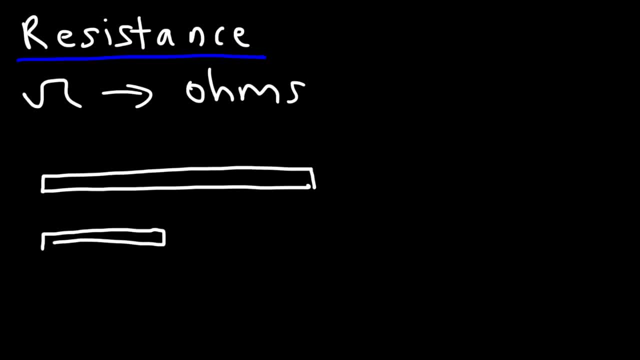 A short wire. Well, you know that a long wire will have more resistance than a short wire because the electrons they have a greater distance to travel through And so longer wires have more resistance than short wires. You have a greater distance to. 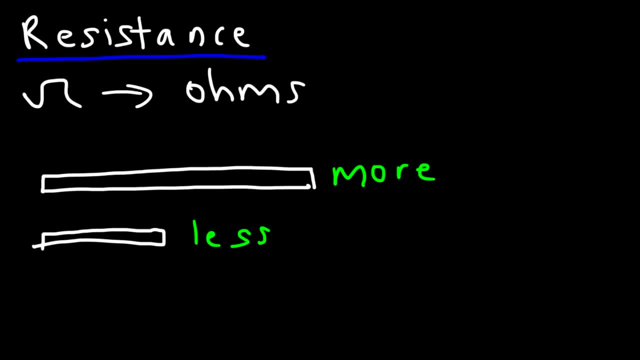 travel to get from one part of the circuit to the other. Now here's another question for you: Which one will have more resistance, A thin wire or a thick wire? It turns out that the thin wire has more resistance than a thick wire And to illustrate this, resistance and current they're inversely related As 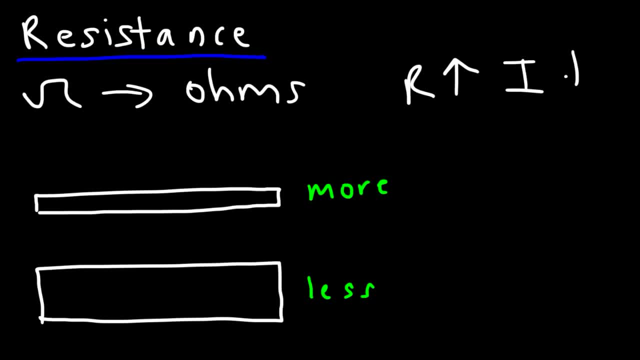 you increase the resistance of a circuit, the current decreases, So the rate at which electrons can travel through the circuit decreases. if you increase the resistance And think of a highway with cars flowing, Think of the cars as being the electrons. In which case will the rate at which cars flow through any given point be greater? Let's 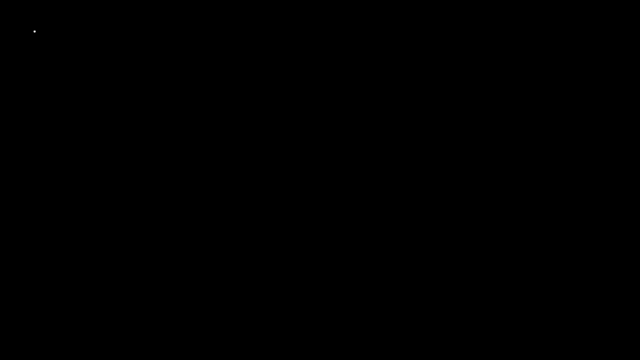 similarities in that instance. Now, the next topic we have is resistance. And when you think of resistance, what do you think of Resistance? they can be used to provide a circuit or devices called resistors, And they resist the flow of current. 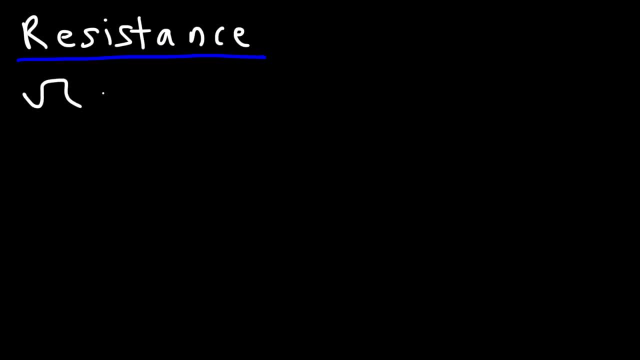 Resistance is measured in the unit's ohms, represented by the Greek symbol omega, And that's basically what you need to know about resistors. They resist the flow of current. Now here's a question for you: Which type of wire will have more resistance? Let's say: 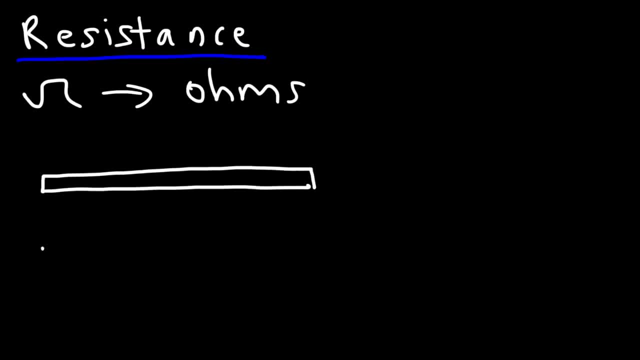 a long wire or a short wire. Which type of wire will have more resistance? Let's say, a long wire or a short wire? Which type of wire will have more resistance? Let's say a long wire or a short wire? Well, you know that a long wire will have more resistance than a short wire, because 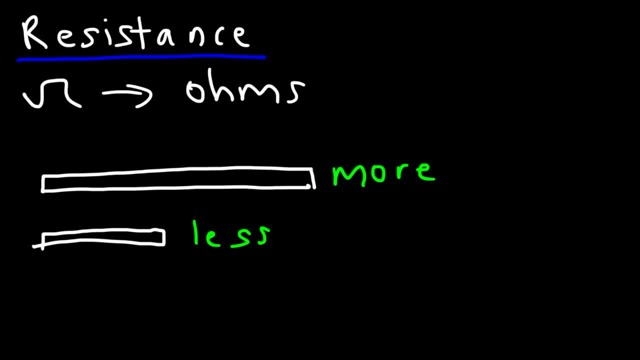 the electrons. they have a greater distance to travel through, And so longer wires have more resistance than short wires. You have a greater distance to travel to get from one part of the circuit to the other. Now here's another question for you, Which one will have. 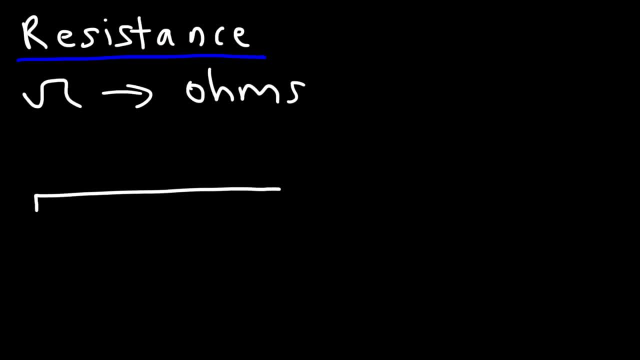 more resistance a thin wire or a thick wire? It turns out that the thin wire has more resistance than a thick wire And to illustrate this, resistance and current: they're inversely related. As you increase the resistance of a circuit, the current 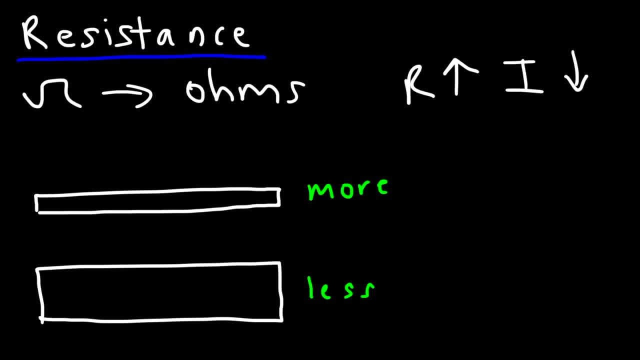 decreases, So the rate at which electrons can travel through the circuit decreases. if you increase the resistance And think of a highway with cars flowing, Think of the cars as being the electrons, In which case will the rate at which cars flow through any given point 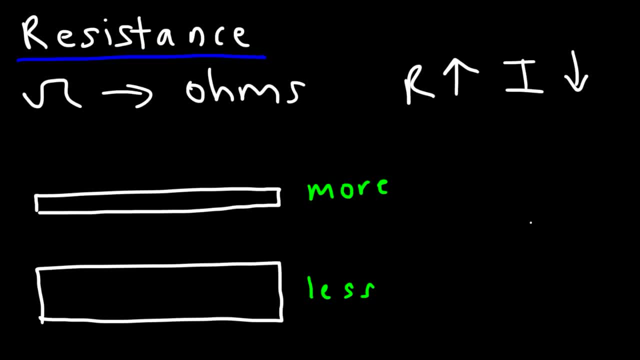 be greater. Let's say, if you have a one-lane highway, or let's say a seven-lane highway. By the way, the green part here represents resistance. It's not current, So just keep that in mind. In a one-lane highway there's not many cars that can get through. 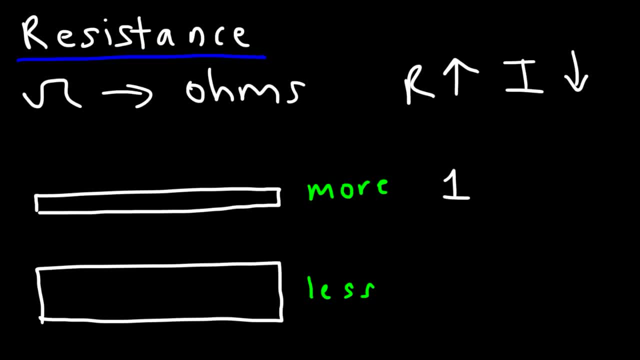 say, if you have a one-lane highway or let's say, a seven-lane highway. By the way, the green part here represents resistance, not current, So just keep that in mind. In a one-lane highway, there's not many cars that can get through, And so the 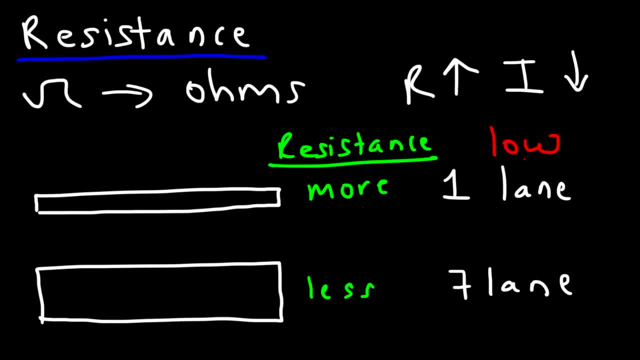 current, which I'm going to highlight in red, will be low in a one-lane highway. However, in a seven-lane highway you can get more cars passing through any given point in a seven-lane highway. So the current will be high but the resistance will be low in a 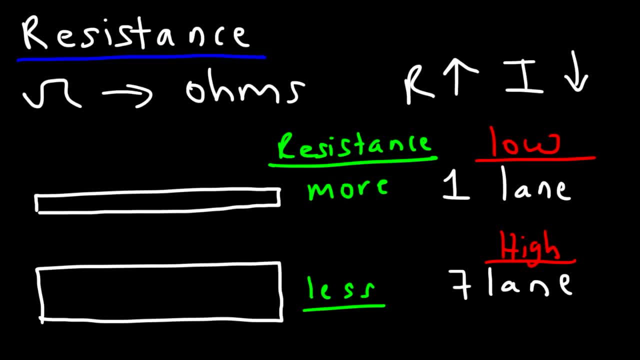 seven-lane highway because a lot of cars can get through, And so the current will be- Think of resistance as being that one-lane highway. The cars are restricted on traveling on that highway, But in a seven-lane highway there's not much resistance. 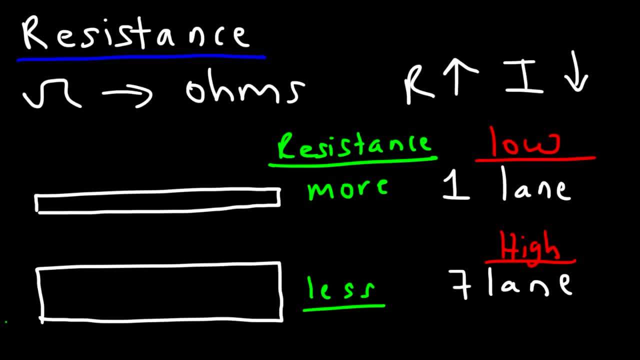 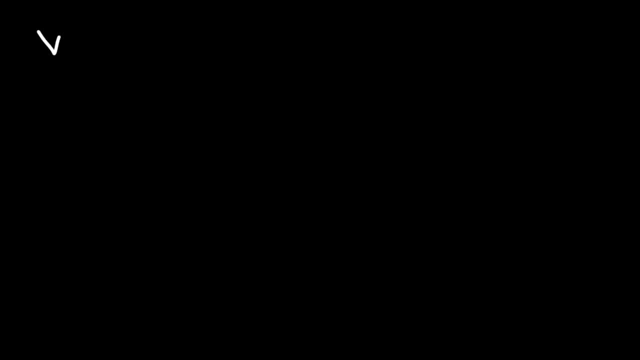 and so you can get a lot of cars, a lot of current flowing through. So keep this in mind. Resistance and current, they are inversely related. Now there is an equation that relates voltage, current and resistance together, And this equation is known as Ohm's Law. 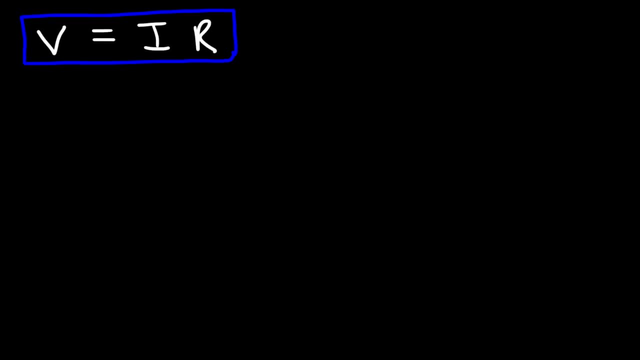 Now let's say, if the resistance is kept constant, What's going to happen to the current in the circuit if we increase the voltage? Increasing the voltage will cause an increase in current. And to illustrate this, imagine if you have, let's say, a pipe that's filled with water. 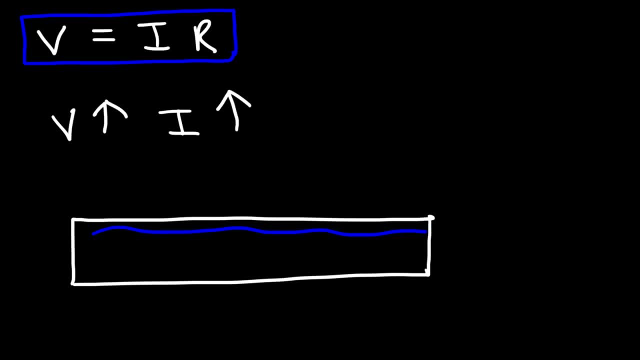 And so you have water in this pipe. Now what's going to happen if you increase the pressure on this circuit? So let's say on the left side the pressure is high And on the right side the pressure is low, But imagine this pipe is completely filled with water. 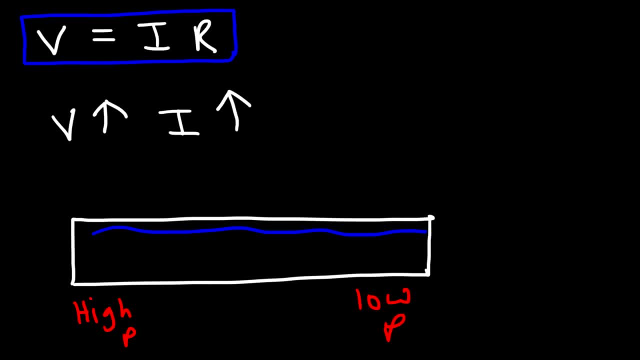 So we really don't have any space here, but it's just filled with water. If the pressure on the left side is high, then the water is going to be forced to move in one direction. It's going to flow from a region of high pressure to 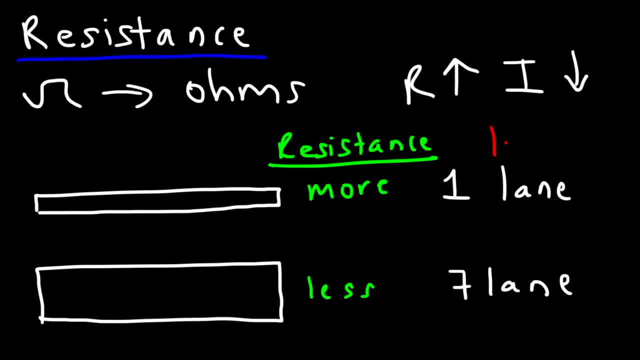 And so the current, which I'm going to highlight in red, will be low. in a one-lane highway, However, in a seven-lane highway, you can get more cars passing through at any given point in a seven-lane highway, So the current will be high, but the resistance. 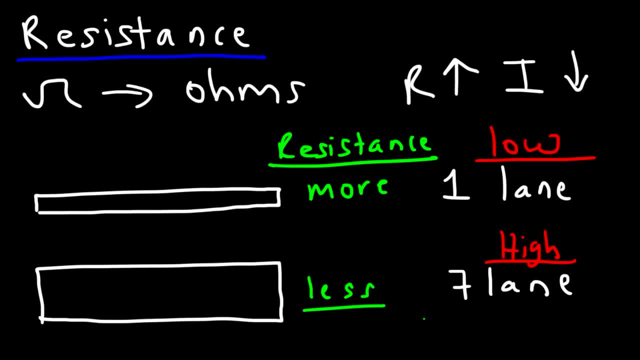 will be low in a seven-lane highway Because a lot of cars can get through, And so think of resistance as being that one-lane highway. The cars are restricted on traveling on that highway, But in a seven-lane highway there's not much resistance And so you can get a lot of cars, a lot of current, flowing through. 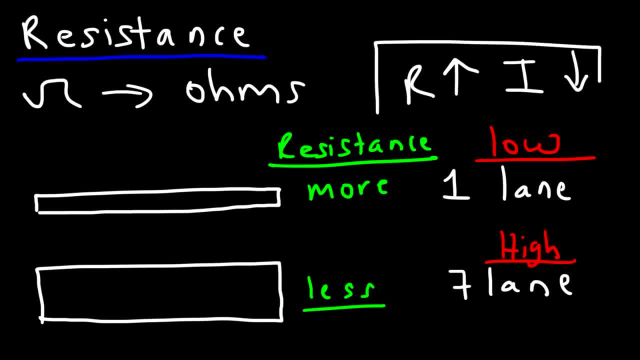 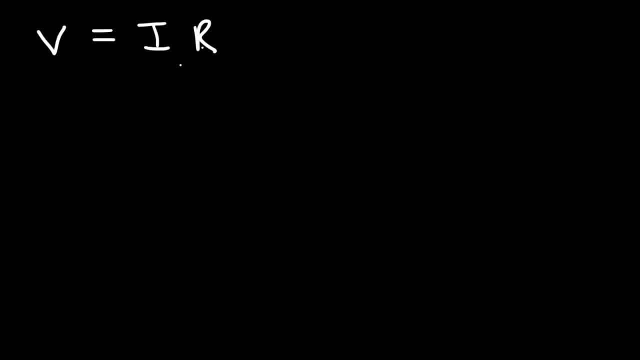 So keep this in mind. Resistance and current, they are inversely related. Now there is an equation that relates voltage, current and resistance together, And this equation is known as Ohm's Law. Now let's say, if the resistance is kept constant, 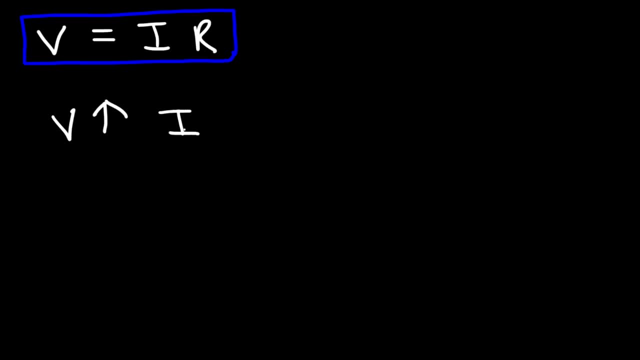 What's going to happen to the current in the circuit if we increase the voltage. Increase in the voltage will cause an increase in current. And to illustrate this, imagine if you have, let's say, a pipe that's filled with water, So you have water in this pipe. 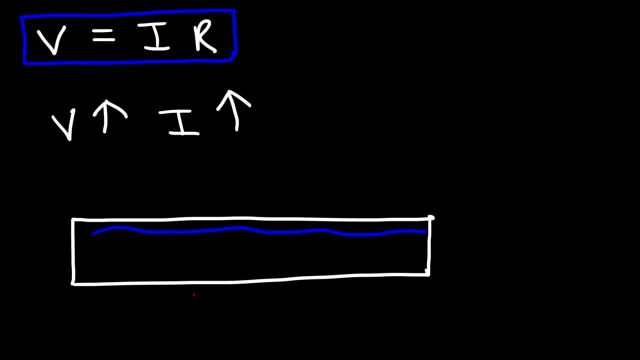 Now what's going to happen if you increase the pressure on this side? So let's say, on the left side the pressure is high And on the right side the pressure is low. But imagine this pipe is completely filled with water. 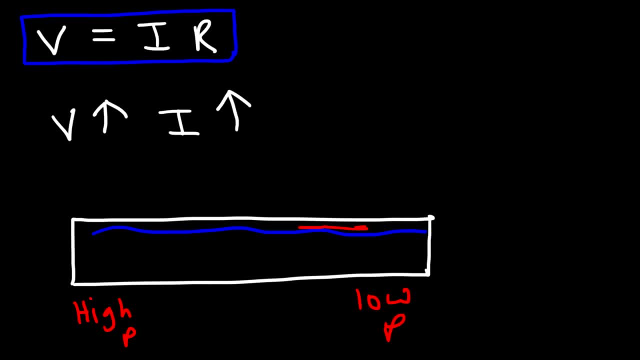 So we really don't have any space here, but it's just filled with water. If the pressure on the left side is high, then the water is going to be forced to move in one direction. It's going to flow from a region of high pressure. 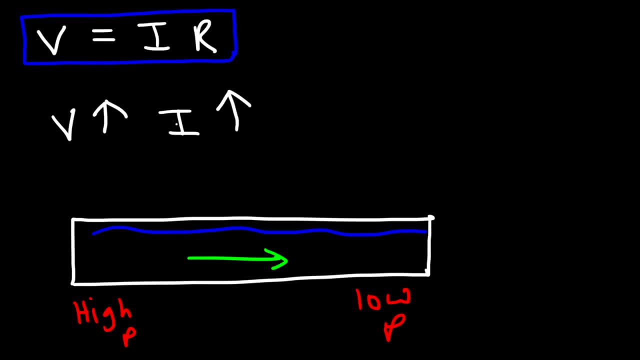 to a region of low pressure, And the same is true with voltage. Current will flow from a region of high voltage to a region of low voltage. So let's say, if the potential on the left side is 10 volts and on the right side the potential is 2 volts, In which 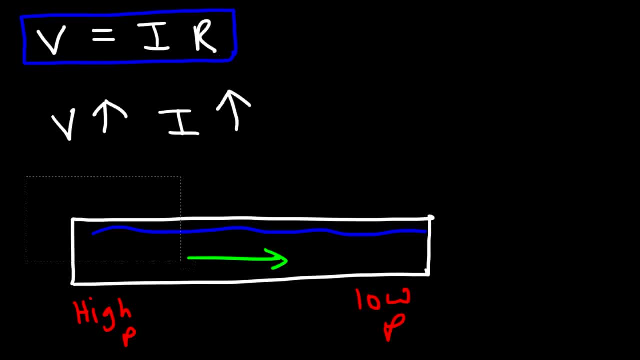 a region of low pressure, And the same is true with voltage. Current will flow from a region of high voltage to a region of low voltage. So let's say, if the potential on the left side is 10 volts and on the right side the potential is 2 volts, 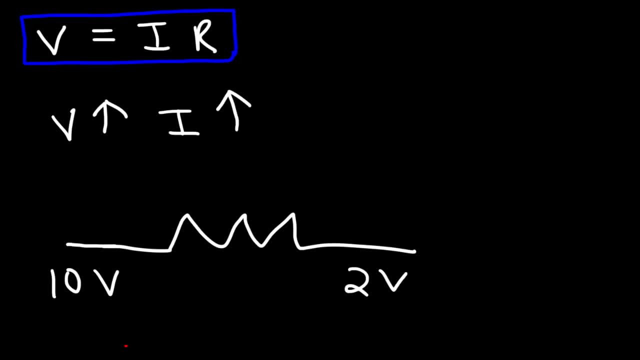 In which direction will the current flow? Well, the voltage is, well the electric potential. rather, It's high on the left side and low on the right side. So the current will flow from a region of high electric potential to a region of low electric potential. 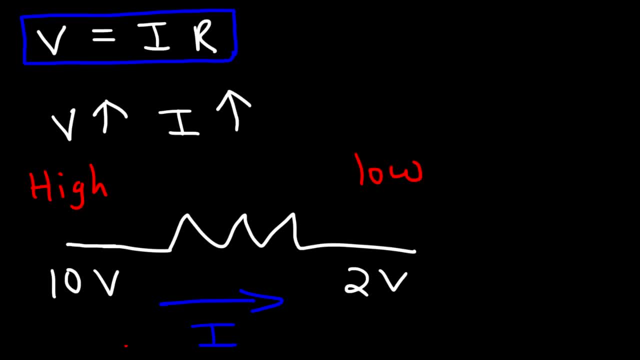 By the way, current and electron flow. they're different. Let's say, if the electrons are flowing in this direction, conventional current is defined as the flow of positive charge, So it's flowing in the other direction. So, even though current flows from high potential to low potential, 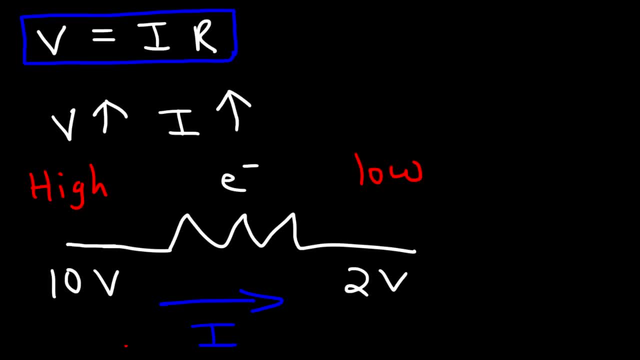 electrons. they flow from low potential to high potential. Electrons are more attracted to a positive charge as opposed to a negative charge, So they're going to flow towards the more positive side. But when dealing with current, I'm going to focus on conventional current, the flow of positive charge. 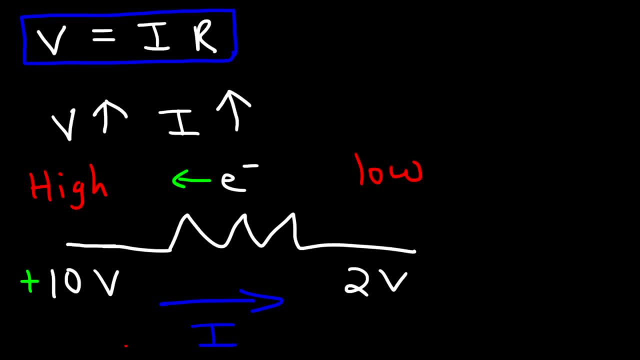 even though negatively charged electrons are flowing in the circuit. Now let me give you another picture. Let's say This is negative 12 volts on the left and negative 18 volts. Let's make it actually. let's make this negative 4 volts on the right. 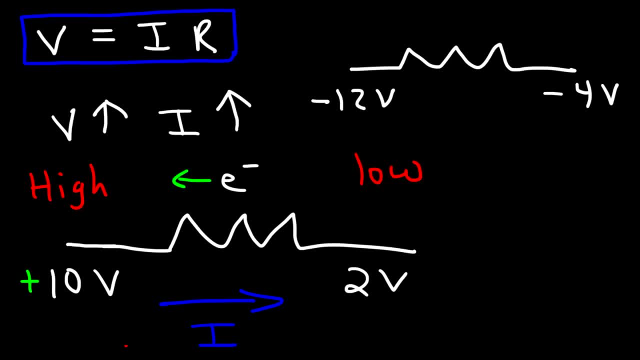 So in which direction is the current flowing, That is, the flow of positive charge? Is it flowing to the right or is it flowing to the left? Feel free to pause the video and think about it Now. which cell, Which side has the high potential and which side has the low potential? 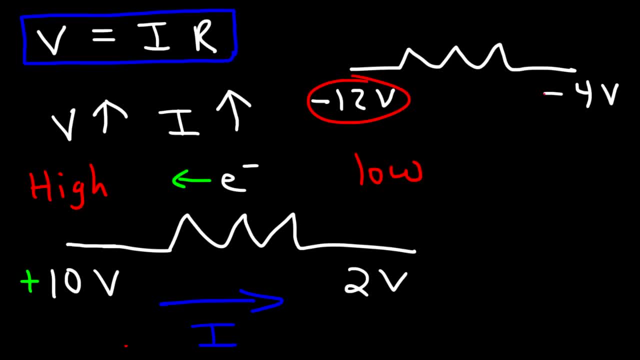 On a number line. which number is greater? Negative 12 or negative 4?? If we draw a number line, let's say this is 0,, this is 5, this would be negative 4, and negative 12 would be somewhere over here. 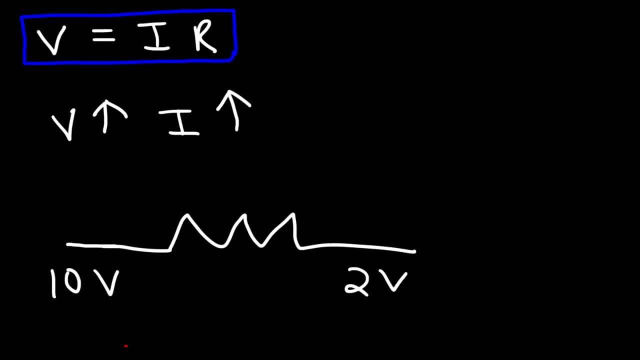 direction will the current flow? Well, the voltage is well, the electric potential, rather, is high on the left side and low on the right side, So the current will flow from a region of high electric potential to a region of low electric potential. By the way, current and 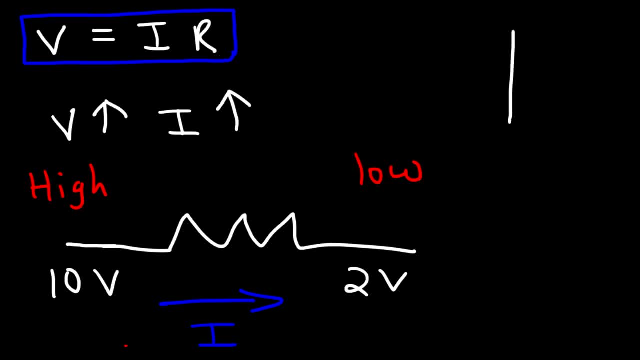 electron flow. they're different. Let's say, if the electrons are flowing in this direction, conventional current is defined as the flow of positive charge, So it's flowing in the other direction. So, even though current flows from high potential to low potential, 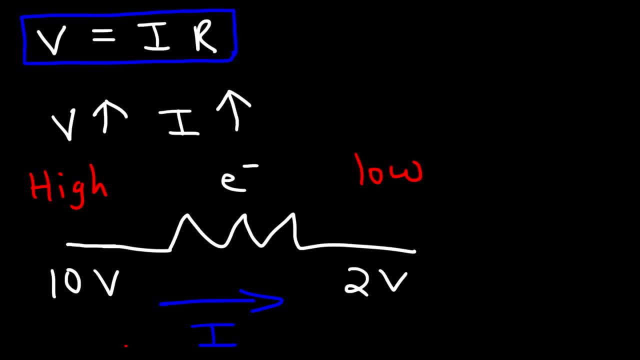 electrons. they flow from low potential to high potential. Electrons are more attracted to a positive charge as opposed to a negative charge, So they're going to flow towards the more positive side. But when dealing with current, I'm going to focus on conventional current, the flow of positive. 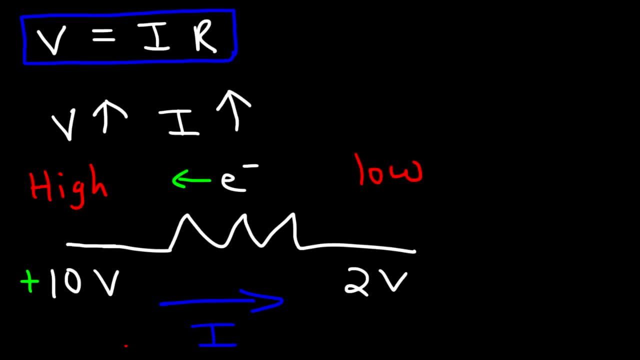 charge, Even though negatively charged electrons are flowing in the circuit. Now let me give you another picture. Let's say this is negative 12 volts on the left and negative 18 volts. Let's make it- uh, actually, let's make this- negative 4 volts on the right. 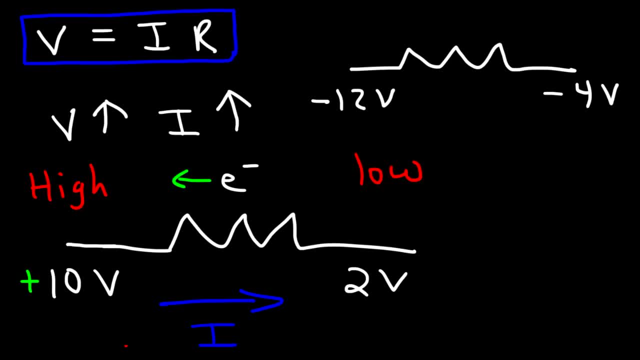 So in which direction is the current flowing, That is, the flow of positive charge? Is it flowing to the right or is it flowing to the left? Feel free to pause the video and think about it Now. which side has the high potential and which side has the low potential On a number line? 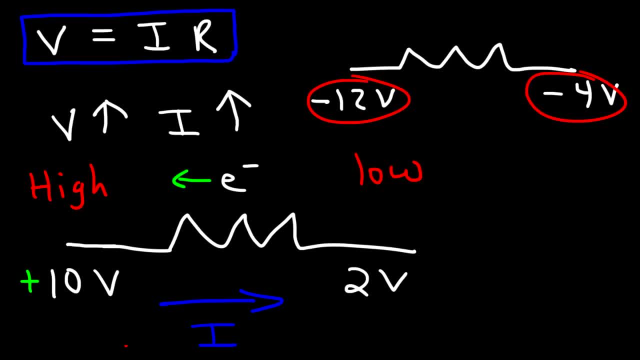 which number is greater: negative 12 or negative 4?? If we draw a number line, let's say this is 0,, this is 5,, this would be negative 4, and negative 12 would be somewhere over here. So the value. 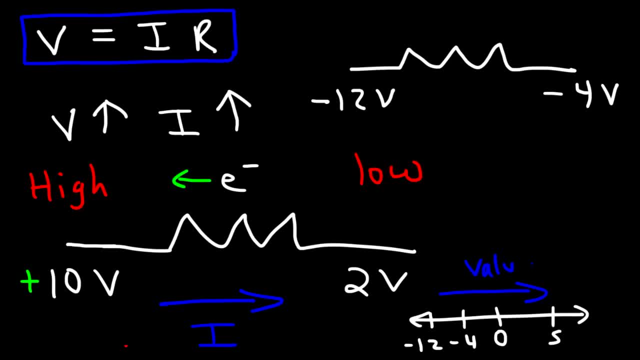 increases as you go towards the right on a number line. So, therefore, negative 4 is higher on a number line than negative 12. And so current is going to flow from a region of high potential to a region of low potential. In this case, it's going to flow towards the left, towards. 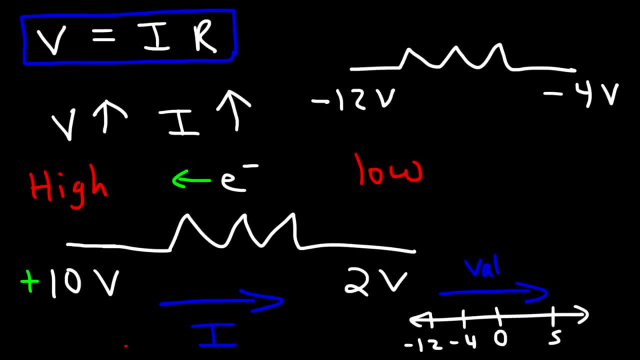 So the value increases as you go towards the right on a number line. So therefore, negative 4 is higher on a number line than negative 12. And so current is going to flow from a region of high potential to a region of low potential. 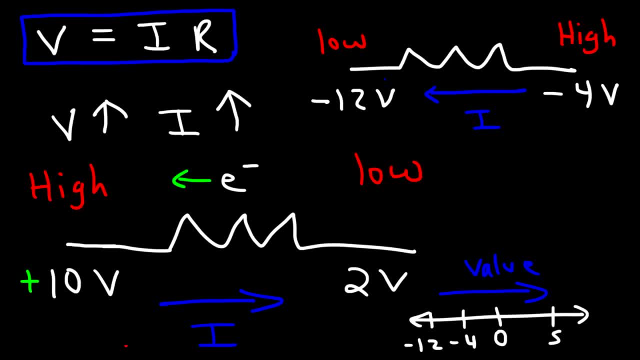 In this case it's going to flow towards the left, towards the lower potential, which is negative 12 volts. So current flows to the more negative side or the less positive side, as in the case of this example. Here, this side is more negative. 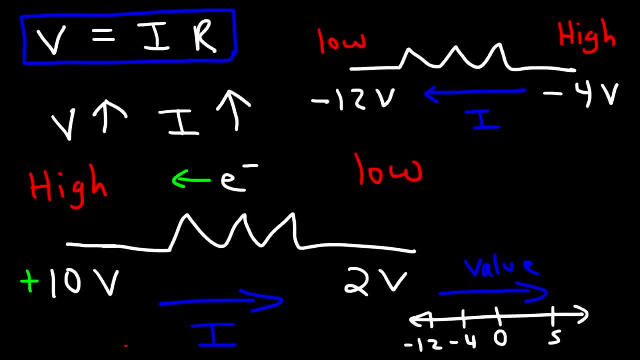 so current is going to flow in that direction. So current flows from high potential to low potential. Now here's a question for you. Let's focus on this picture. What is the voltage across the resistor? You need to understand the difference. 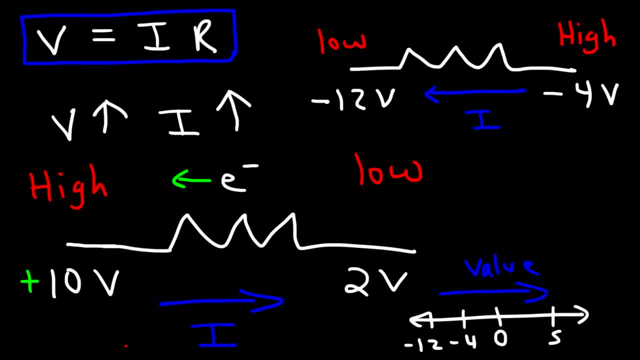 between electric potential and voltage. Now let's call this point point A and this point point B. Now the electric potential at point A is positive 10 volts. The electric potential at point B is 2 volts. Voltage is the difference between the electric potentials. 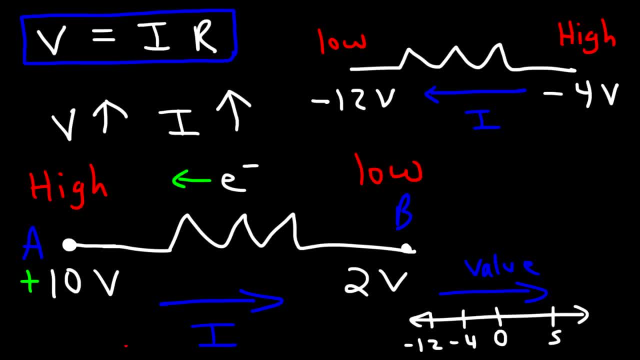 of two points. So it's the electric potential difference of two points. So the voltage across the resistor is the difference between A and B. So in that case the voltage across that resistor- we can call it Vr- It's 8 volts. 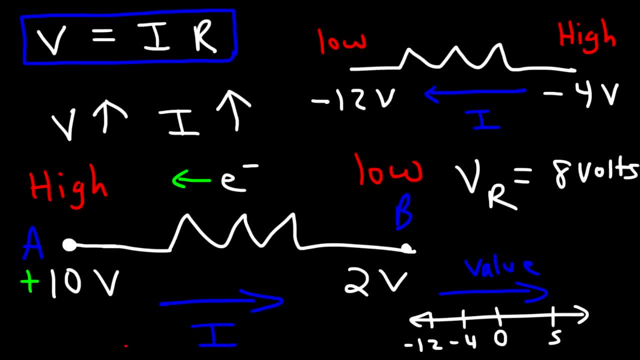 It's the difference between those two points. Now, what about the voltage across this resistor? It's also 8 volts. Now, sometimes this could be negative 8, depending on how you connect it. So let's say, if you connect the positive terminal, 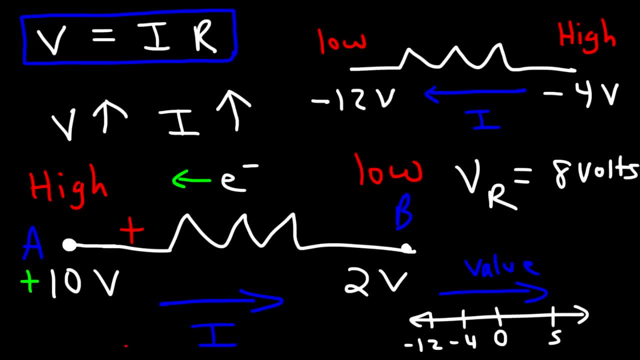 of, let's say, a meter to point A and the negative terminal to point B, it's going to read: positive 8.. However, if you connected the negative terminal of a meter to point A and a positive terminal of the meter to point B, the current 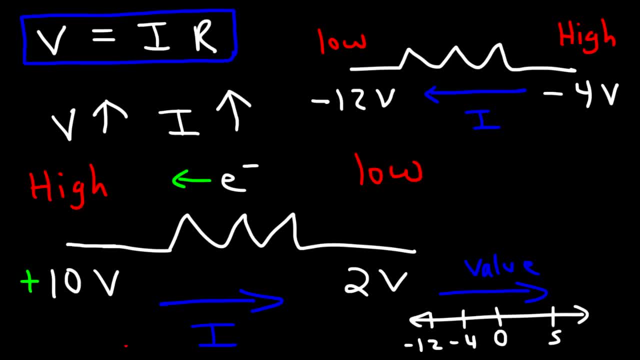 the lower potential, which is negative 12 volts. So current flows to the more negative side or the less positive side, as in the case of this example. Here this side is more negative, so current is going to flow in that direction. So current flows from high potential to low potential. 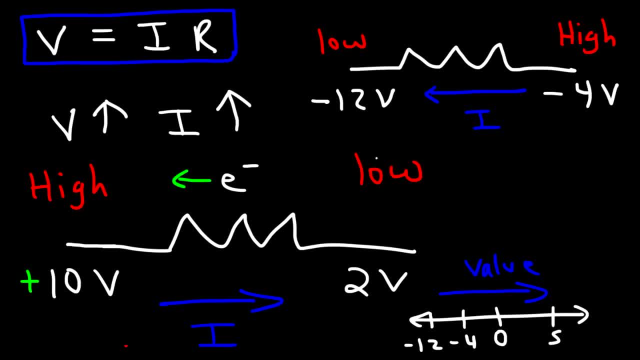 Now here's a question for you. Let's focus on this picture. What is the voltage across the resistor? You need to understand the difference between electric potential and voltage. Now let's call this point point A and this point point B. 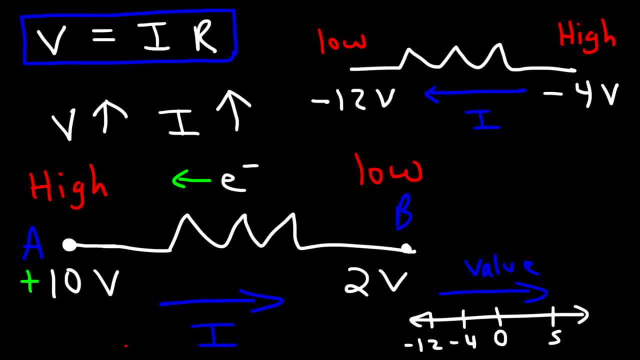 Now the electric potential at point A is positive 10 volts. The electric potential at point B is 2 volts. Voltage is the difference between the electric potentials of two points. So it's the electric potential difference of two points, So the voltage across the resistor. 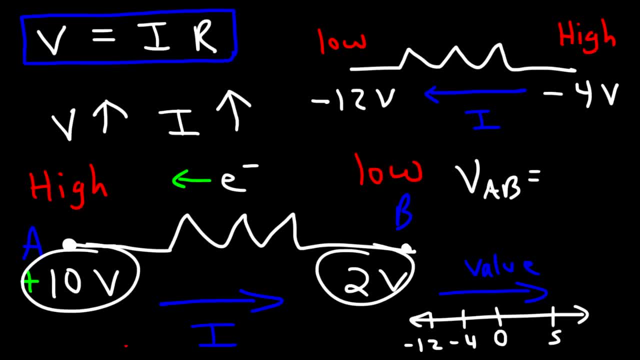 is the difference between A and B. So in that case, the voltage across that resistor- we can call it Vr- is 8 volts. It's the difference between those two points. Now, what about the voltage across this resistor? It's also 8 volts. 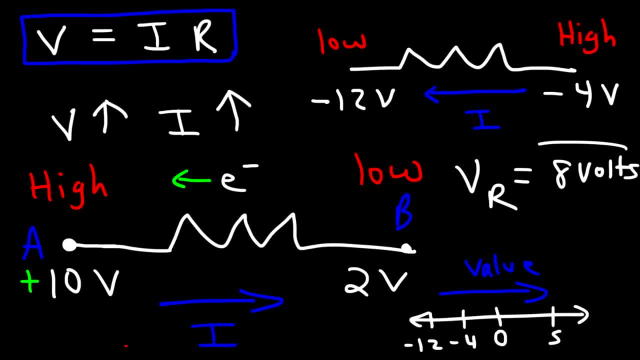 Now, sometimes this could be negative 8, depending on how you connect it. So let's say, if you connect the positive terminal of, let's say, a meter to point A and the negative terminal to point B, it's going to read: 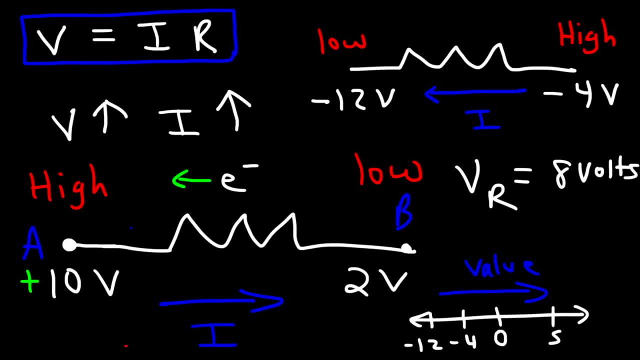 positive 8 volts. However, if you connected the negative terminal of a meter to point A and the positive terminal of the meter to point B, the current will basically be reversed in that meter, And so the voltage that it's going to read will be negative 8.. So, depending on the way you connect it, 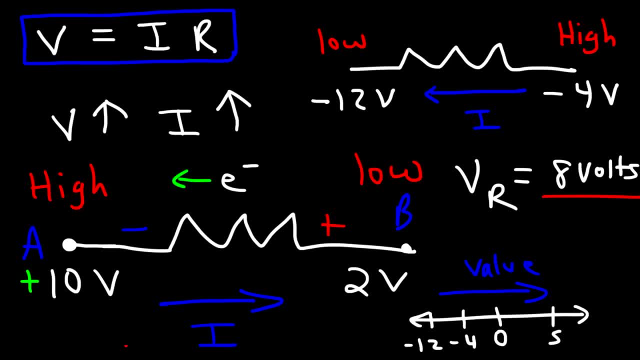 you can get a reading of positive 8 or negative 8.. But if you want to get a positive reading, connect the positive terminal to the high potential part of the circuit and the negative terminal to the low potential part of the circuit, And then you'll get a positive reading. 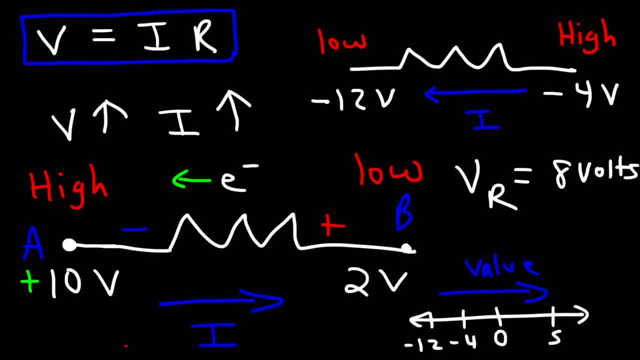 will basically be reversed in that meter, And so the voltage that it's going to read will be negative 8.. So depending on the way you connect it, you can get a reading of positive, 8 or negative 8.. But if you want to get a positive reading, 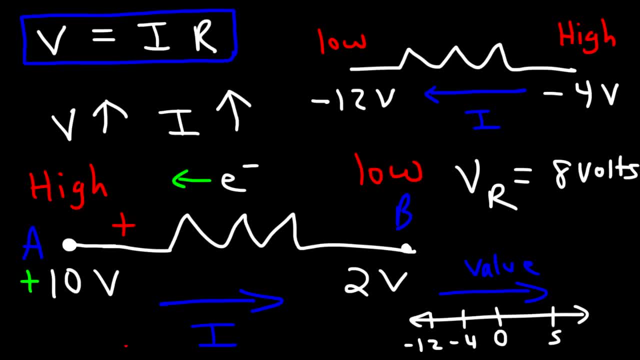 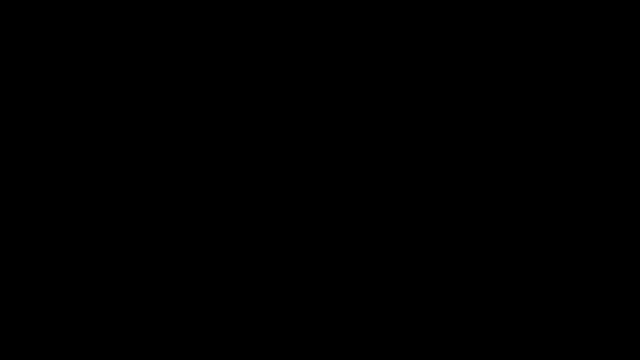 So that's what we're going to do, And then you'll get a positive reading. Now let's go back to this. So we said that if we increase the voltage in a circuit, the current will increase, And also if you increase the resistance of a circuit, 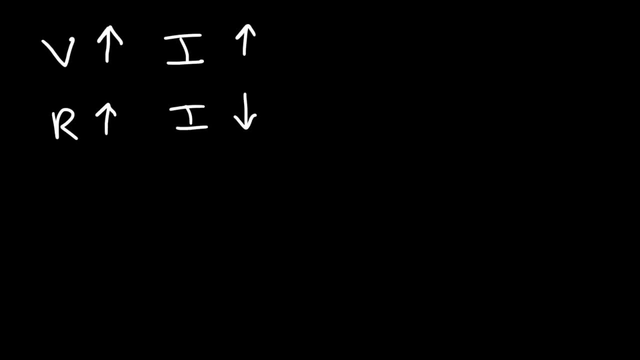 the current will decrease. So make sure you understand these statements from Ohm's law. So voltage is directly related to current and resistance is inversely related to current. So if you double the voltage in a circuit, with everything else being the same, 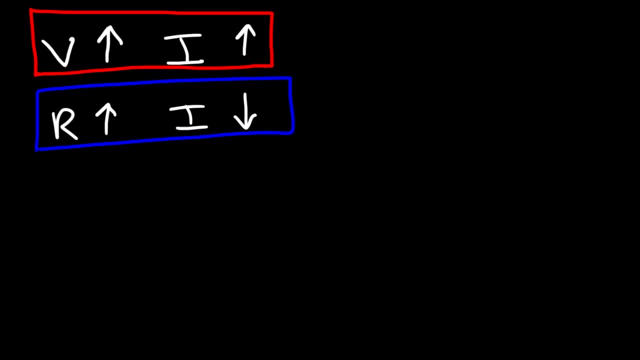 the current will double. If you double the resistance, the current will reduce by a factor of 2. It will be half of what it used to be. If you triple the voltage, the current will triple. If you triple the resistance, the current will be one-third of its original value. 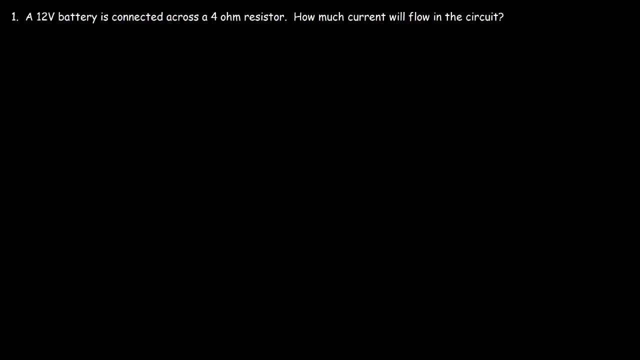 Now let's work on some practice problems. A 12-volt battery is connected across a 4-ohm resistor. How much current will flow in the circuit? So this is the electrical symbol of a battery. And let's draw the electrical symbol of a resistor. 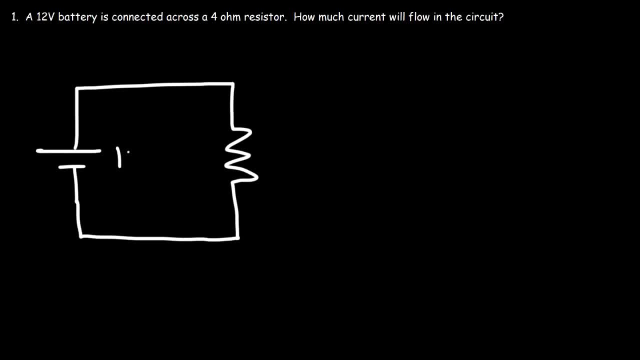 which looks like that, And so this is a 12-volt battery And we have a 4-ohm resistor. Now this is the negative terminal of the battery and this is the positive terminal, So current will flow from the positive terminal to the negative terminal. 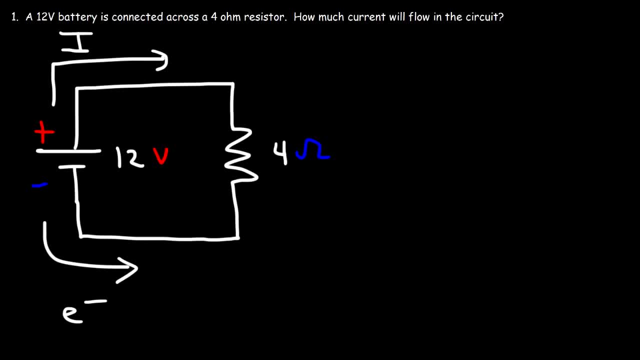 But keep in mind the electrons are flowing in the opposite direction. Now, using Ohm's Law, V is equal to IR. we can get the answer. I like using it in this form because I can easily solve for any variable that I need. 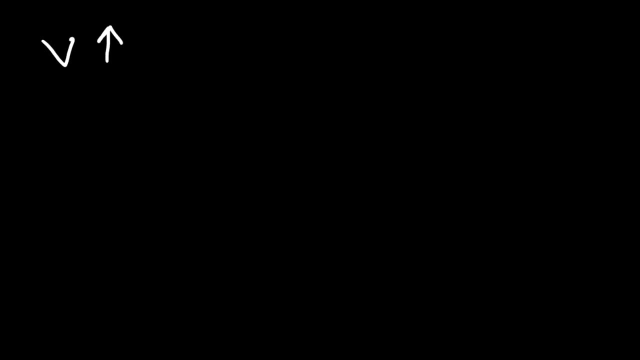 Now let's go back to this. So we said that if we increase the voltage in a circuit, the current will increase, And also if you increase the resistance of a circuit, the current will decrease. So make sure you understand these statements. 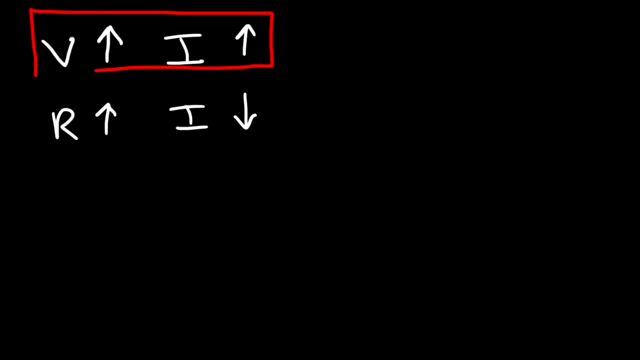 from Ohm's Law. So voltage is directly related to current and resistance is inversely related to current. So if you double the voltage in a circuit, with everything else being the same, the current will double. If you double the resistance, the current will. 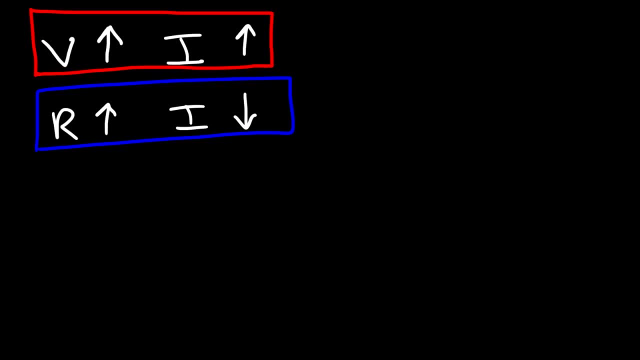 reduce by a factor of 2. It will be half of what it used to be. If you triple the voltage, the current will triple. If you triple the resistance, the current will be 1 third of its original value. Now let's work on some practice problems. 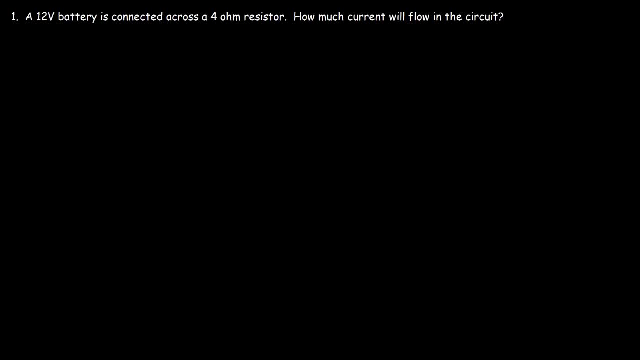 A 12 volt battery is connected across a 4 ohm resistor, How much current will flow in the circuit? So this is the electrical symbol of a battery, And let's draw the electrical symbol of a resistor which looks like that. And so this is a 12 volt battery. 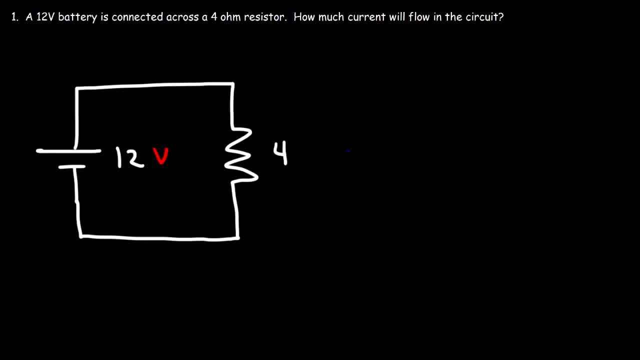 and we have a 4 ohm resistor. Now this is the negative terminal of the battery and this is the positive terminal. So current will flow from the positive terminal to the negative terminal, But keep in mind the electrons are flowing in the opposite direction. 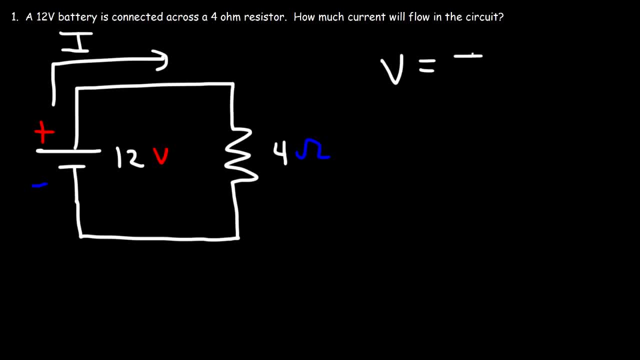 Now, using Ohm's law, V is equal to IR, we can get the answer. I like using it in this form because I can easily solve for any variable that I need just using some simple algebra. So the voltage is 12, the current in the circuit is what we're looking for. 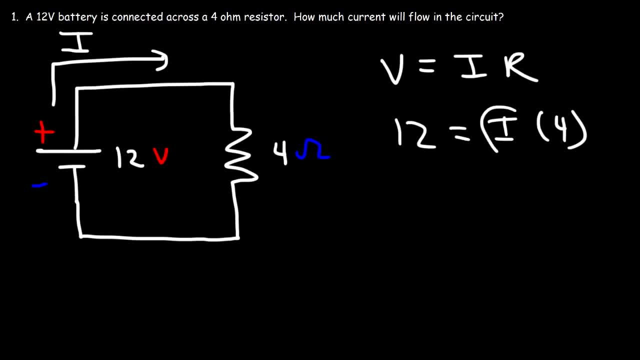 and the resistance is 4.. So to get I by itself to solve for the value of I, I need to divide both sides by 4.. On the right side, 4 divided by 4 is 1, giving me just I. 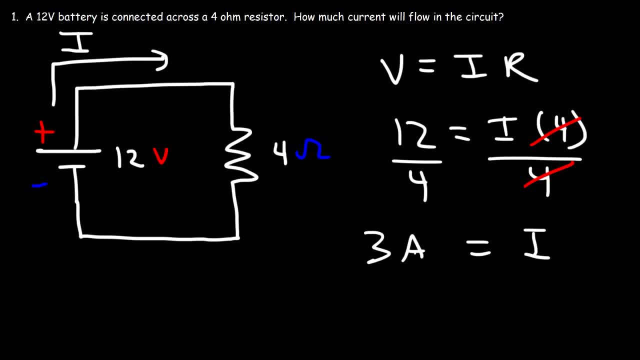 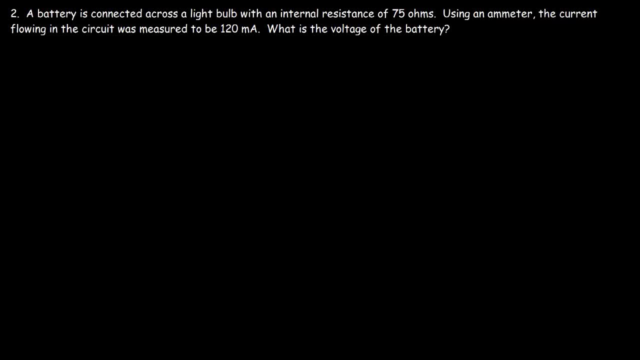 On the left side, 12 divided by 4 is 3.. Thus the current in the circuit is 3 amps, And that's the answer Number 2.. A battery is connected across a light bulb with an internal resistance of 75 ohms. 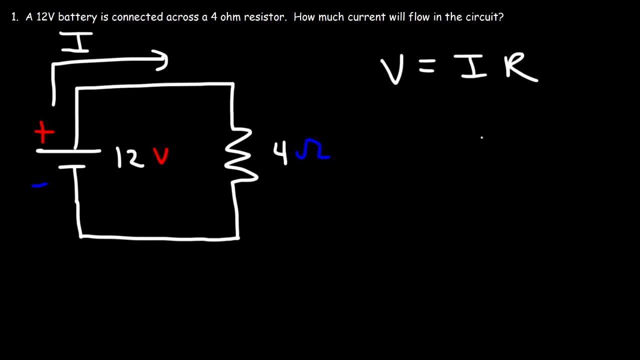 just using some simple algebra. So the voltage is 12.. The current in the circuit is what we're looking for and the resistance is 4.. So to get I by itself to solve for the value of I, I need to divide both sides by 4.. 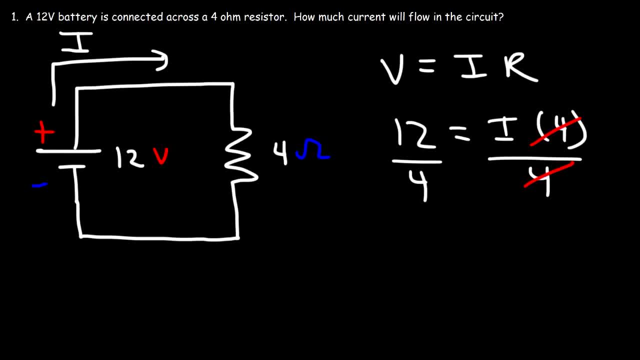 On the right side, 4 divided by 4 is 1,, giving me just I. On the left side, 12 divided by 4 is 3.. Thus the current in the circuit is 3 amps And that's the answer. 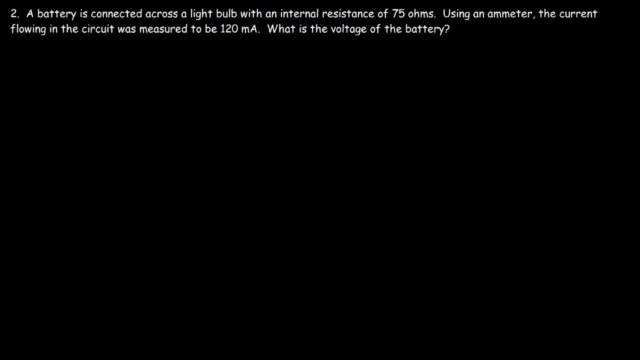 Number 2.. A battery is connected across a light bulb with an internal resistance of 75 ohms. Using an ammeter, the current flowing in the circuit was measured to be 120 milliamps. If you see mA, that's milliamps. 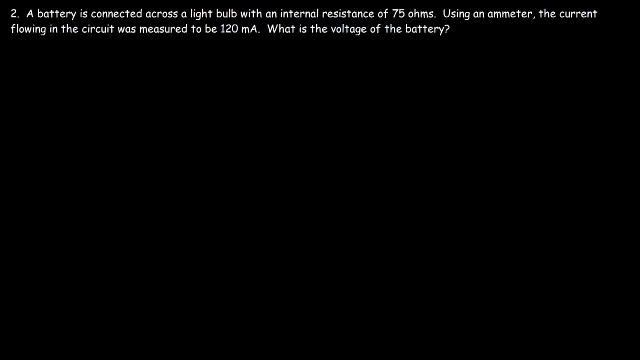 What is the voltage of the battery. So feel free to pause the video and draw a circuit with the appropriate elements and then solve it. Now let's start with the battery. So here's the battery And here is the ammeter. You can just put an A in a circle. 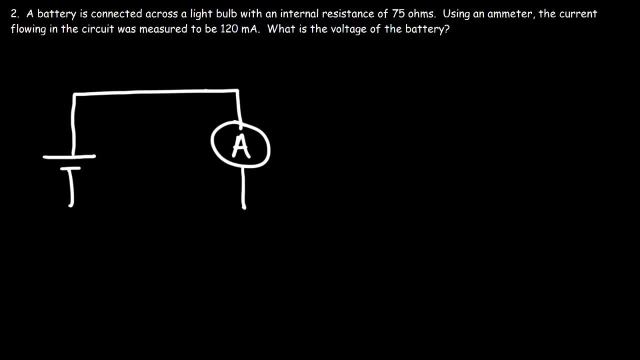 And then let's draw the light bulb, which this is one way you can draw the light bulb, Or you can draw a light bulb like this, if you want, And let's turn the light bulb on. So what is the voltage of the battery? 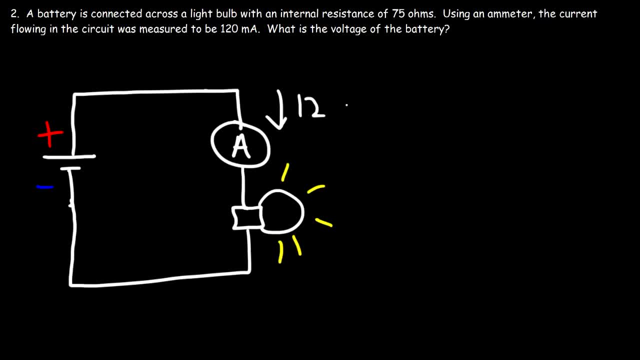 Now the ammeter detects a current of 120 milliamps. How can we convert that to amps? Now it's important to understand that one amp is equal to a current of 1000 milliamps, So to convert milliamps to amps. 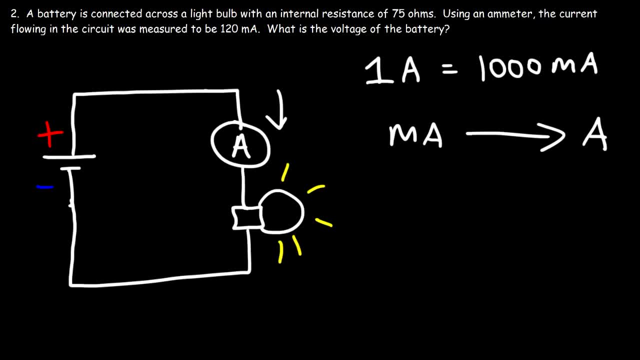 you need to divide by 1000. So if we take 120 and divide it by 1000, all we need to do is take the die and divide it by 1000. So if we take 120 and divide it by 1000, all we need to do is take the die and divide it by 1000.. 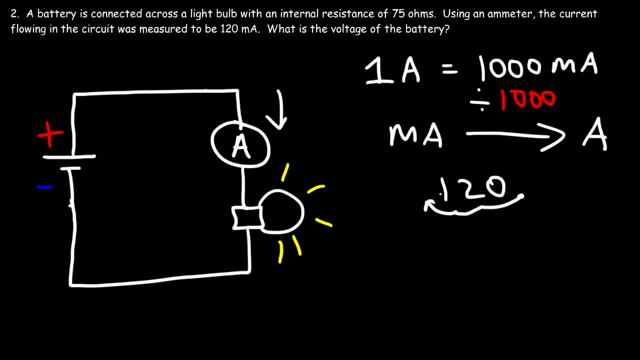 All we need to do is take the decimal point and move it three spaces to the left, And that will give us a current of 0.12 amps, And so that's a quick way in which you can convert milliamps to amps. 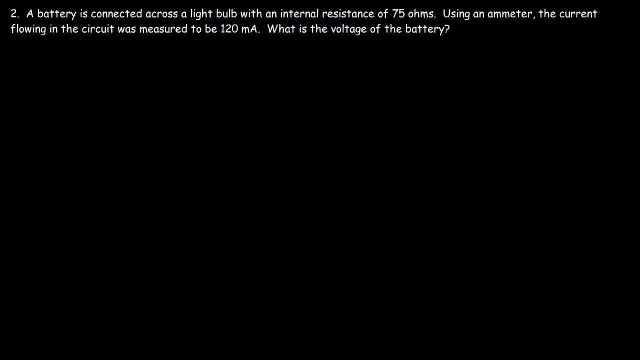 Using an ammeter, the current flowing in the circuit was measured to be 120 milliamps, What is the voltage of the battery. So feel free to pause the video and draw a circuit with the appropriate elements and then solve it. Now let's start with the battery. 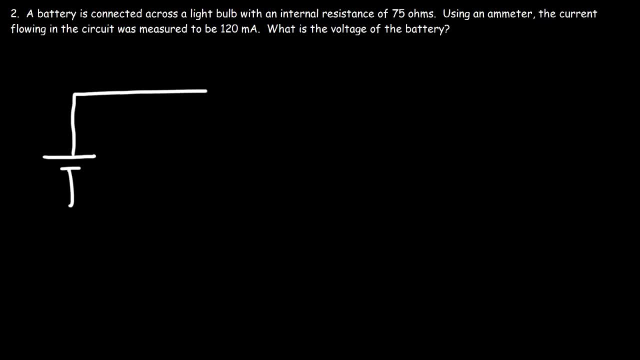 So here's the battery and here is the ammeter. You can just put an A in a circle and then let's draw the light bulb, which this is one way you can draw the light bulb, Or you can draw a light bulb like this, if you want. 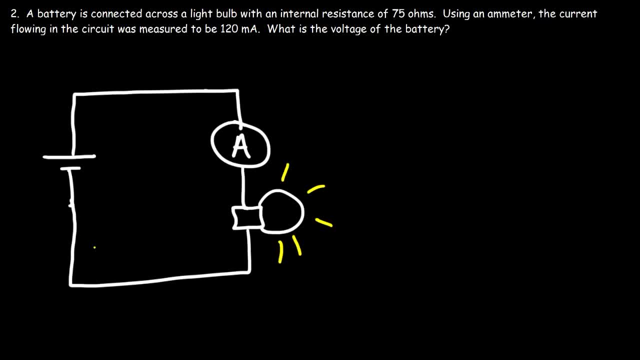 And let's turn the light bulb on. So what is the voltage of the battery Now? the ammeter detects a current of 120 milliamps. How can we convert that to amps Now? it's important to understand that 1 amp is equal to a current of 1000 milliamps. So to convert milliamps to amps you need to divide by 1000. So if we take 120 and divide it by 1000, all we need to do is take the decimal point and move it three spaces to the left And that will give us a current of 0.12. 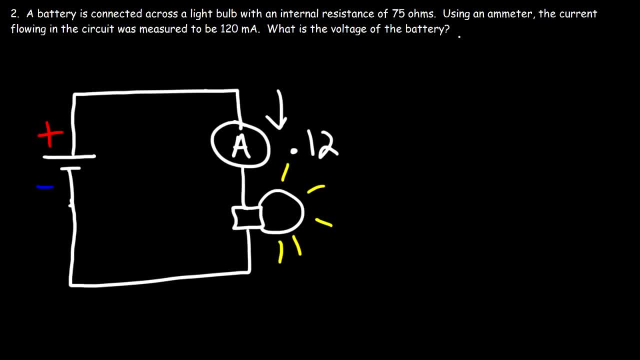 amps, And so that's a quick way in which you can convert milliamps to amps. Now the resistance of the light bulb. we said it was 75 ohms, So now we have everything that we need in order to calculate the voltage of the battery. 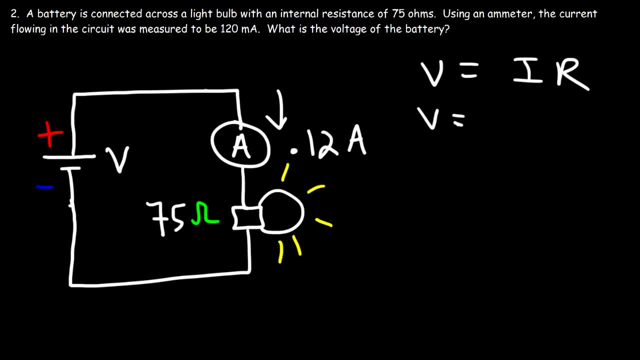 So V equals IR, So the current is 0.12,, the resistance is 75, and so we just need to multiply those two, So 0.12 times 75, what we have is a 9 volt battery. So whenever you're using Ohm's Law, 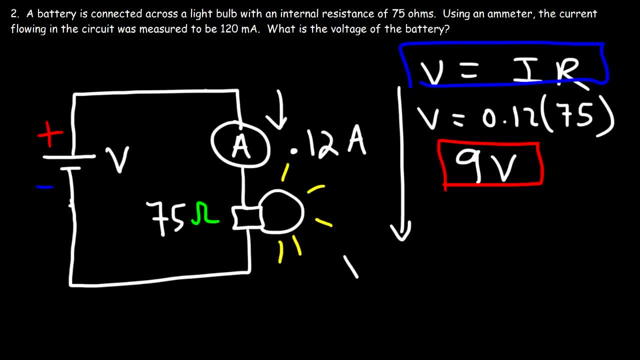 just remember: if V is in volts, then the current has to be in amps and the resistance has to be in ohms. Let's say, if the resistance was in ohms but if you plug in milliamps instead, then this will give you millivolts. 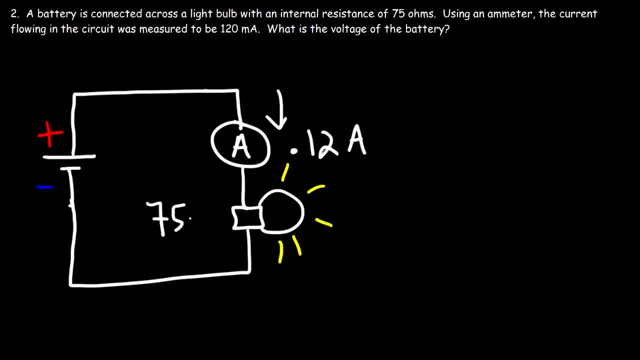 Now the resistance of the light bulb. we said it was 75 ohms, So now we have everything that we need in order to calculate the voltage of the battery. So V equals ir, So the current is 0.12.. The resistance is 0.21. 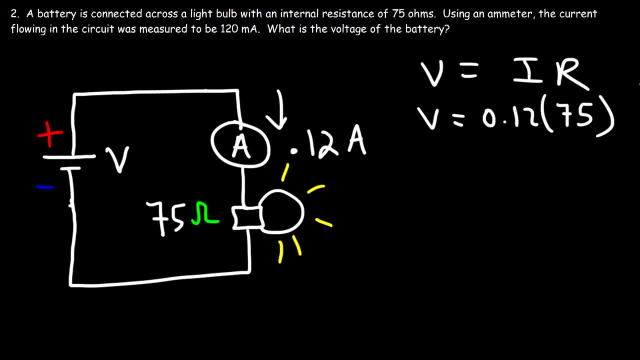 is 75, and so we just need to multiply those two, so point 12 times 75. what we have is a 9 volt battery. so whenever you're using Ohm's law, just remember: if V is in volts, then the current has to be in amps and the resistance has to be in. 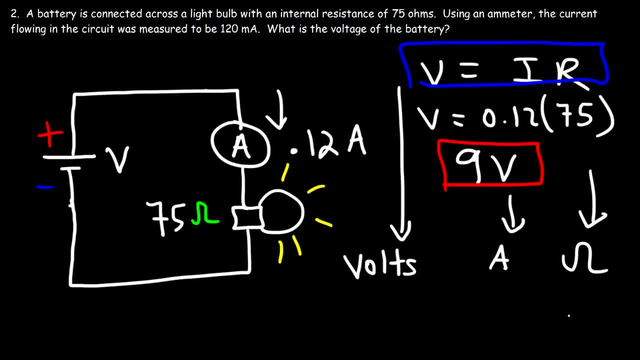 ohms. let's say if the resistance was in ohms, but if you plug in milliamps instead, then this will give you millivolts. so you have to be careful when you're using different units. but just to be on the safe side, use volts. 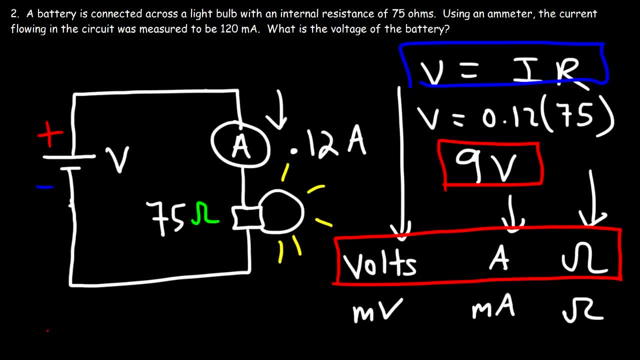 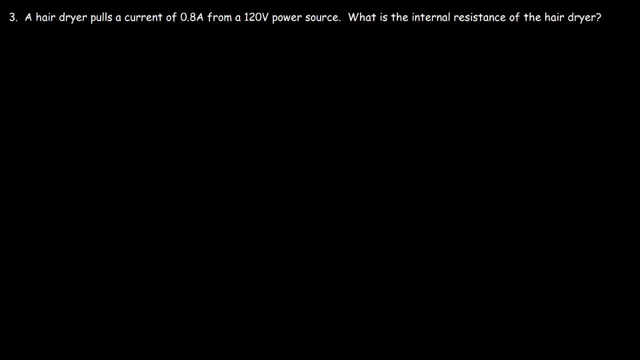 for V amps for the current and ohms for the resistance. number three: a hairdryer pulls a current of 0.8 amps from a 120 volt power source. what is the internal resistance of the hairdryer? so let's go ahead and go. 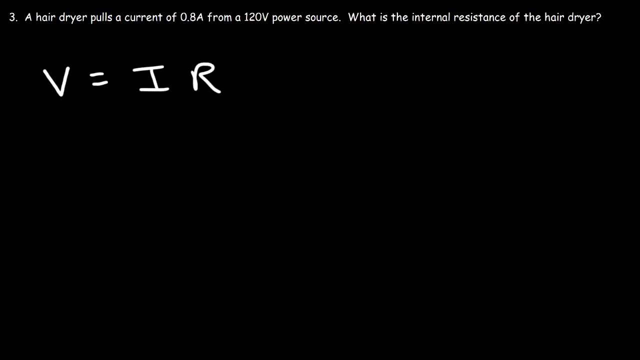 directly to the formula. V equals IR. so we have the voltage, it's 120 volts. we have the current 0.8 amps and our goal is to solve for R the internal resistance of the hairdryer. so V is 120, the current is 0.8 and let's calculate R. 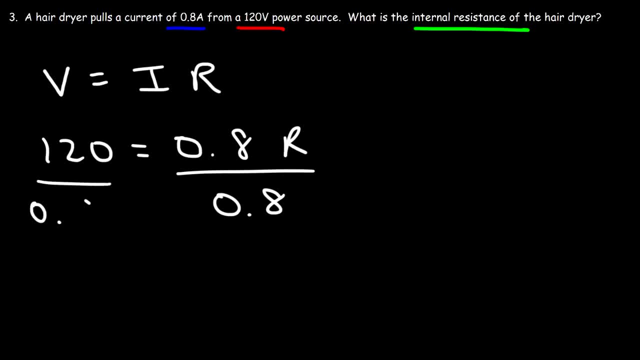 so to get R by itself, we just need to divide both sides by 0.8- you, and so 120 divided by 0.8 is 150, and so the answer is 150 ohms, and that's the resistance of the hairdryer, and so it's very simple to use Ohm's law. 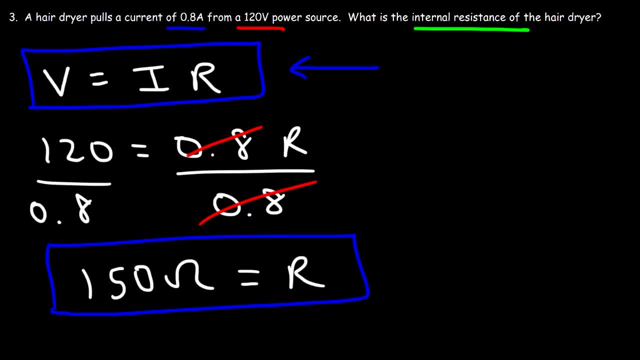 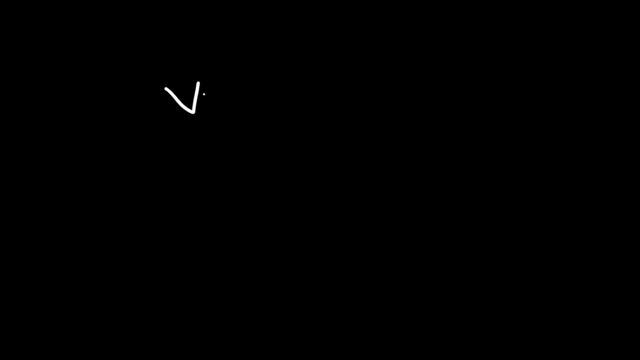 particularly in this format, you can easily calculate the voltage, the current or the resistance. now perhaps you've seen this symbol before, maybe like a triangle or something with V on top and I and R on the bottom. So let's say, if you wish to calculate R, 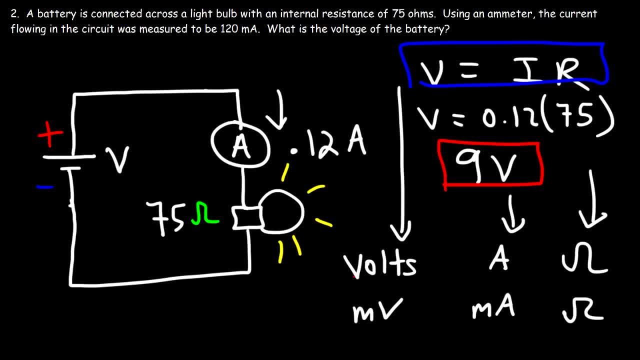 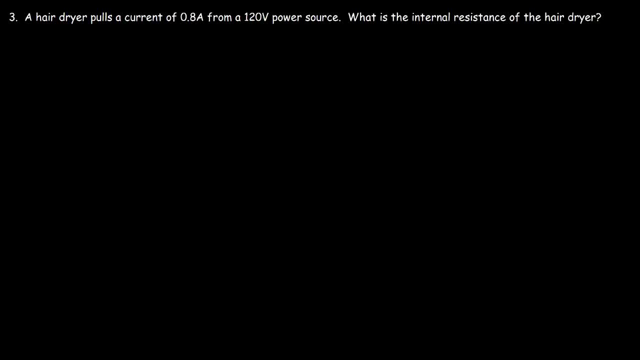 So you have to be careful when you're using different units. but just to be on the safe side, use volts for V, amps for the current and ohms for the resistance. Number three: a hair dryer pulls a current of 0.8 amps. 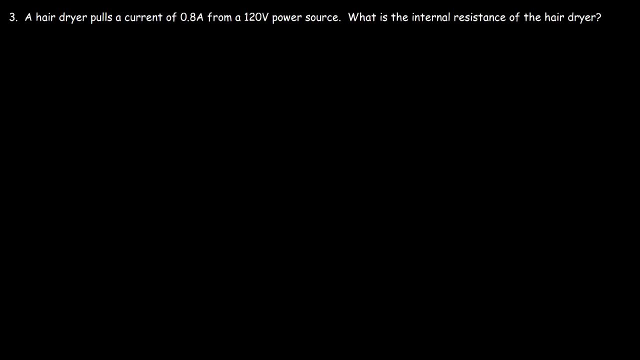 from a 120 volt power source. What is the internal resistance of the hair dryer? So let's go ahead and go directly to the formula. V equals IR. So we have the voltage, it's 120 volts, we have the current 0.8 amps and our goal is to solve for R. 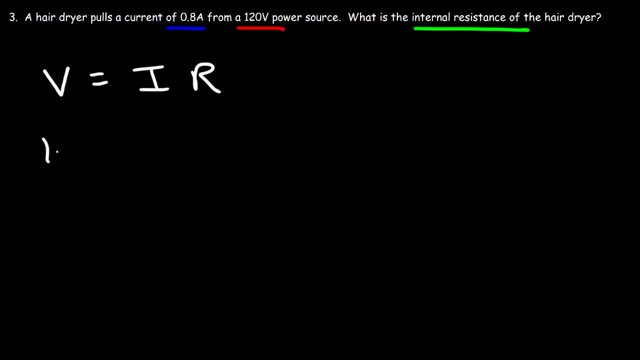 the internal resistance of the hair dryer. So V is 120,, the current is 0.8, and let's calculate R. So to get R by itself, we just need to divide both sides by 0.8.. And so 120. 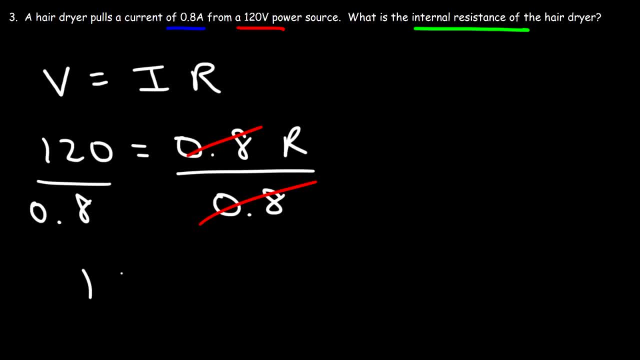 divided by 0.8 is 150.. And so the answer is 150 ohms, And that's the resistance of the hair dryer. And so it's very simple to use Ohm's Law, particularly in this format. You can easily calculate the voltage. 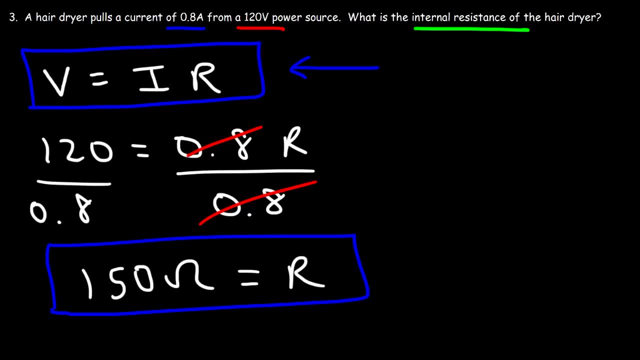 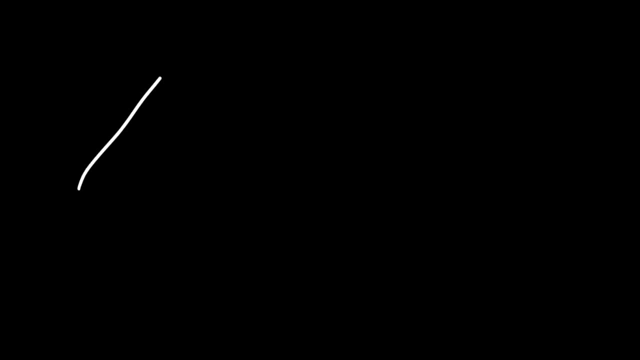 the current or the resistance. Now, perhaps you've seen this symbol before, maybe like a triangle or something, with V on top and I and R on the bottom. So let's say, if you wish to calculate R, Looking at the stuff that's left over. 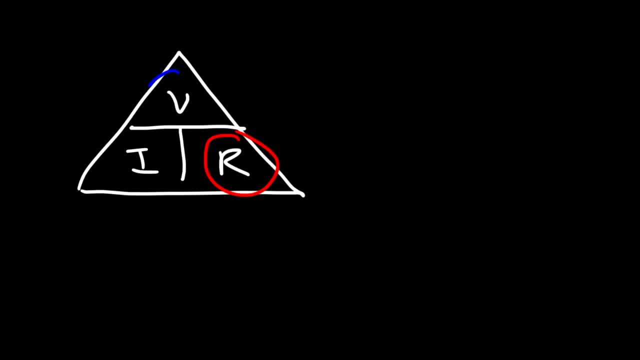 let's say, if you put your thumb on R, you can see that the resistance is voltage divided by current. Now let's say, if you block off the current, If you put your thumb on the current, you can see that the current is voltage divided by resistance. 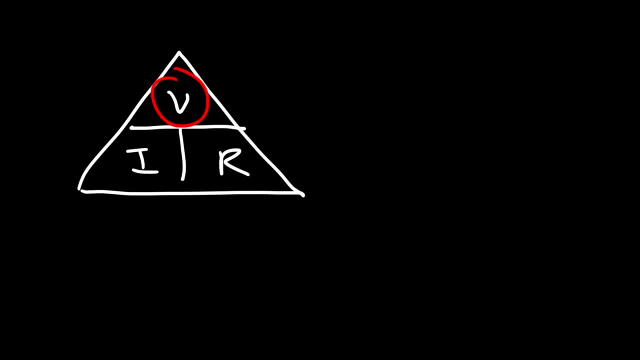 Now, if you put your thumb on, let's say the voltage, then that tells you that voltage is current times resistance, Which we could see in this form. But let's say, if you divide by I, the voltage divided by current is equal to resistance. if you need to calculate R, Or if you need to calculate current,